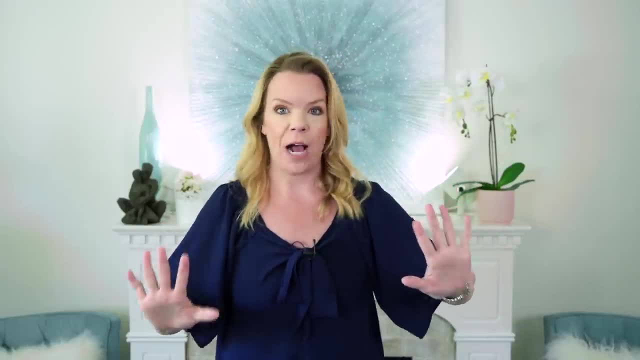 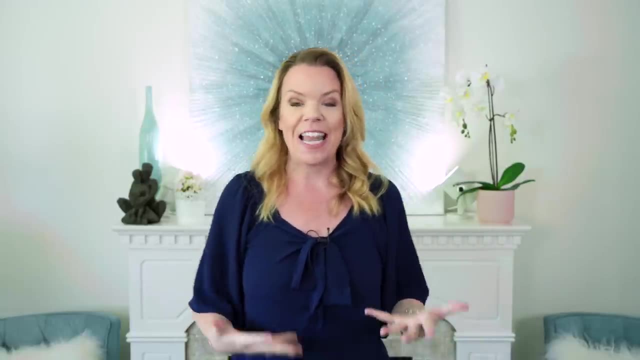 feeling energized. We're going to do this weird thing right now. I need you to stand up. I know this. This is why I don't share it with you, because it's embarrassing. but I need you to stand up, wherever you're watching this, and actually give this a try. There's science behind it. 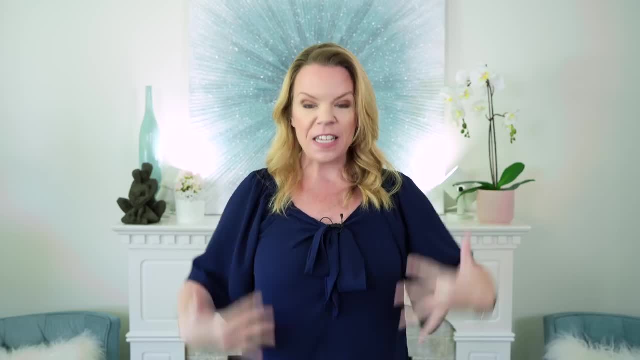 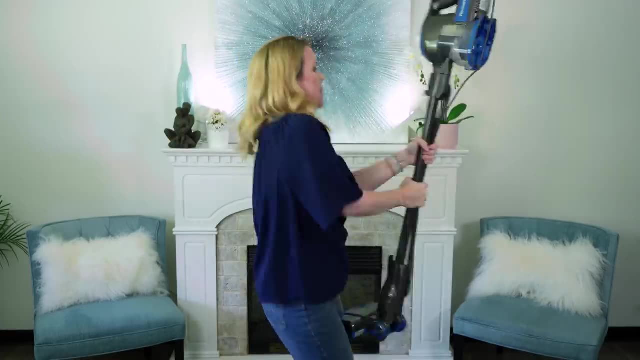 but changing your state means that you're physically feeling and making the motions that you would feel if you were excited about what you were doing. We're faking it. So imagine for a second: I came into your home and completely cleaned and organized everything. 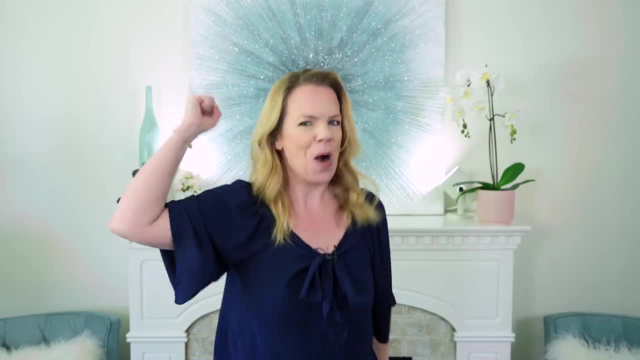 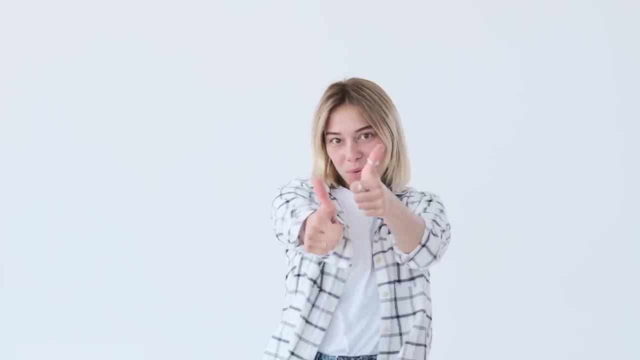 What would you feel like? How would your body react? You'd be like maybe you do jumping jacks. Some people clap, Some people make the motions with their body that they feel when they're excited, So like: can we fist pump, Can we finger guns? I don't know. We're doing something. We're 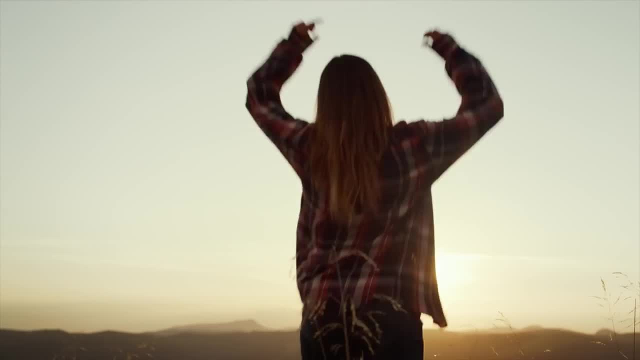 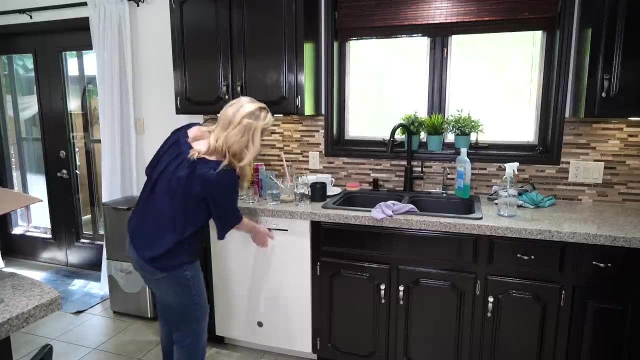 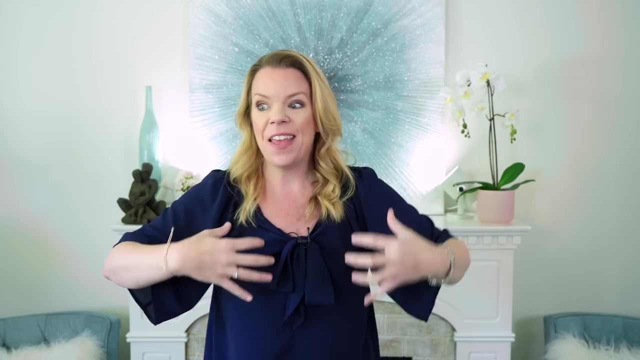 bouncing on our toes, Even if you're just clapping your hands. When I do this, I instantly feel motivated and excited to clean my house. Anytime I look at a sink full of dirty dishes or laundry piled on the floor, I feel defeated, Like my energy gets sucked down, And then I definitely don't feel. 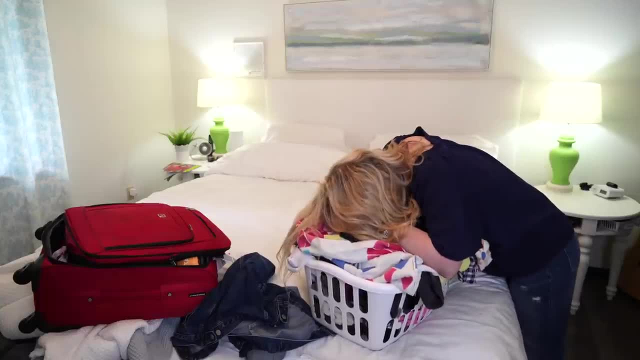 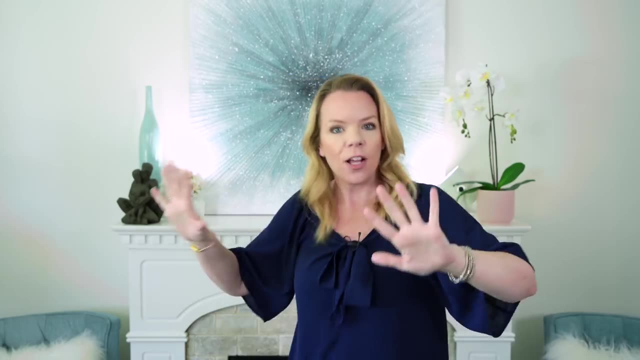 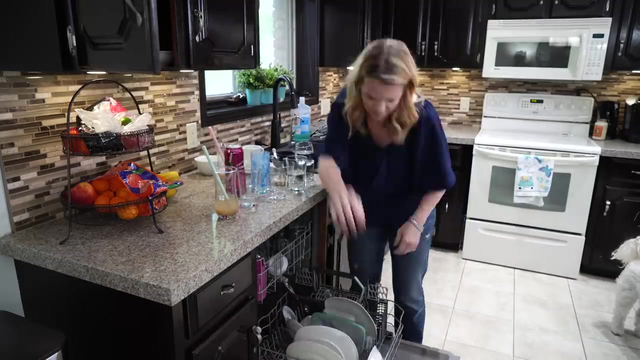 anything. We don't do things or want to do things if we're not feeling excited about it. but we can trick our bodies And there was like a bunch of science-y reasons And I glossed over that part and I tuned out. But basically your body and your brain don't know the difference. So if you're like 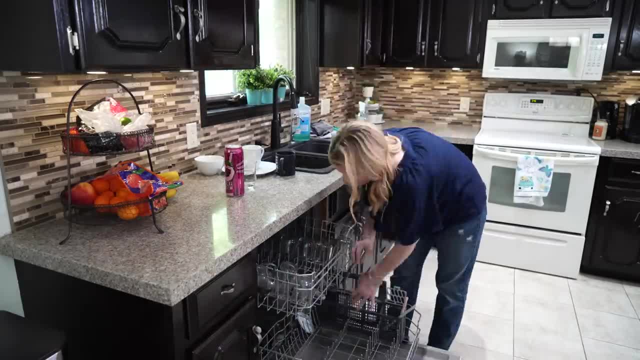 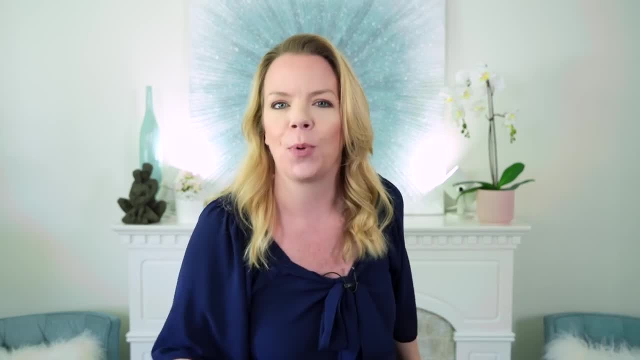 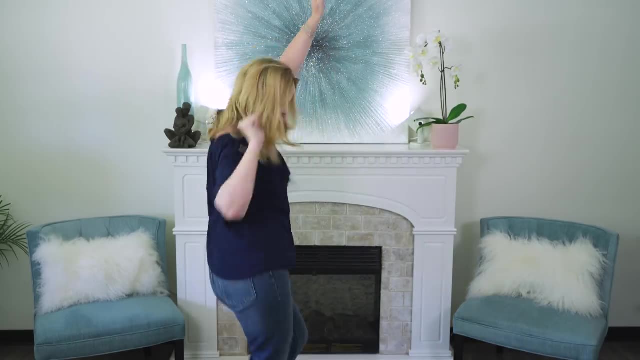 wooing with your body. your brain starts sending you chemicals that you would feel if you were genuinely excited about something, if you were genuinely motivated. So we can fake our brain out to clean the house. I hope you're doing it. Do some like wooing motions right now And the 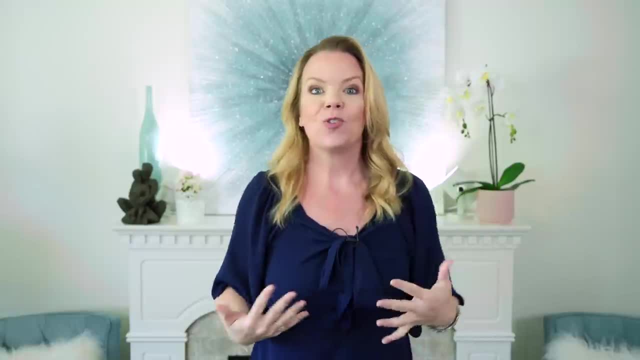 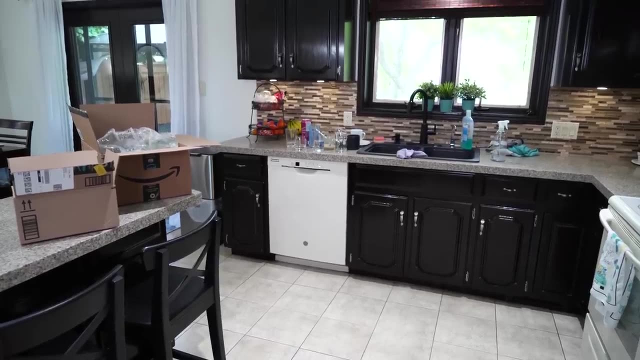 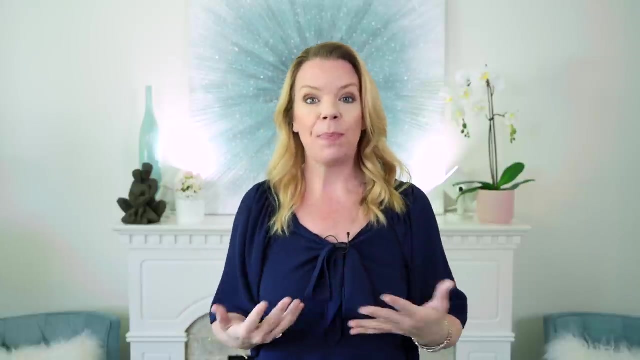 second part. the second trick is story, And this is something that we tell ourselves often: Ugh, I have to clean the kitchen, I don't want to do the dishes, Because the truth is we don't really want to do the dishes. But we can instantly change this a little bit by saying: I get to have a clean. 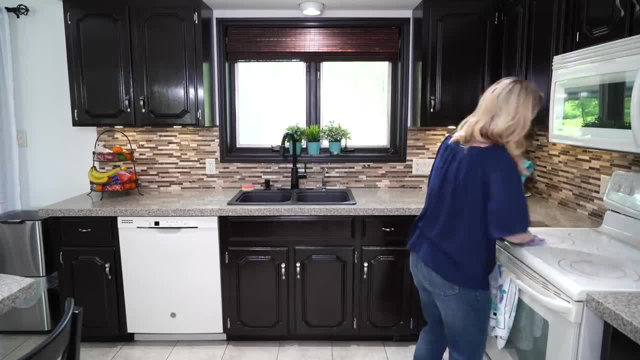 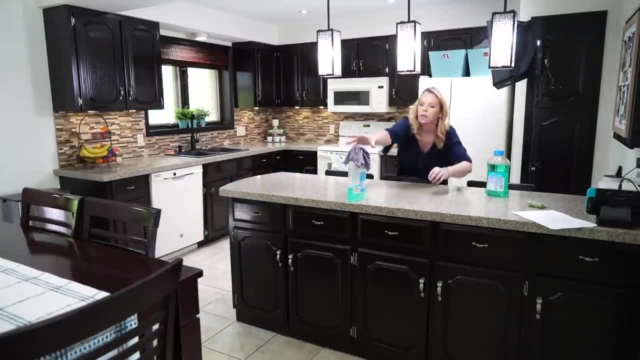 house: no dirty dishes in the sink. I deserve to have a house that doesn't look like a hot mess sandwich. I deserve a clean house. I want you to say that. I want you to say I deserve a clean house. I'm going to give myself a clean house, And you have to say it out loud- which, again? 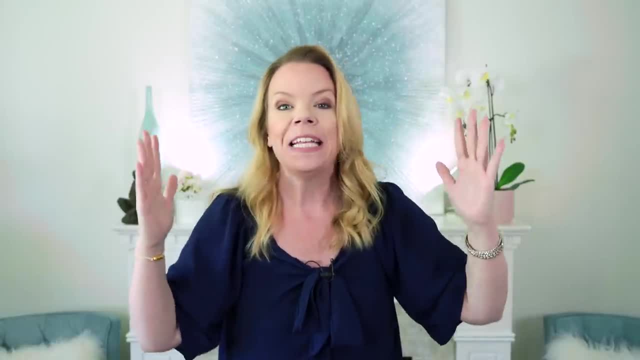 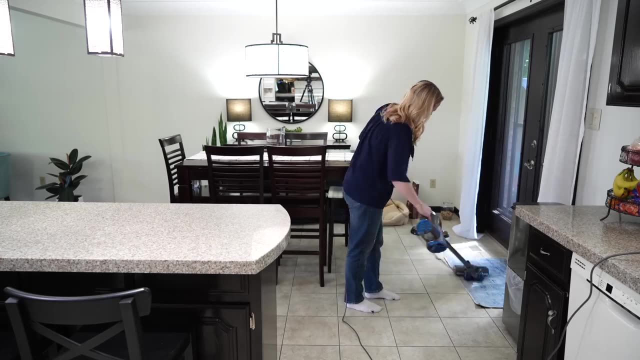 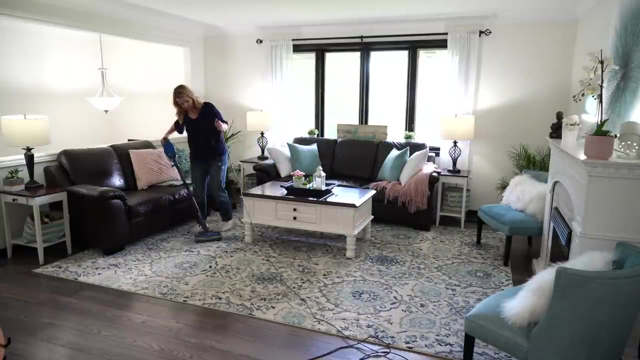 is a little bit embarrassing, but nobody's seeing you. I'm doing this in front of you. I can't see you. I know it's embarrassing, I know it feels uncomfortable, But this works. Okay, it does. It works. You're changing your state, You're changing your story. You're. 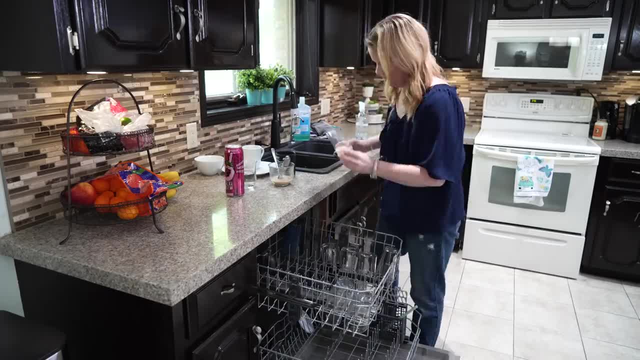 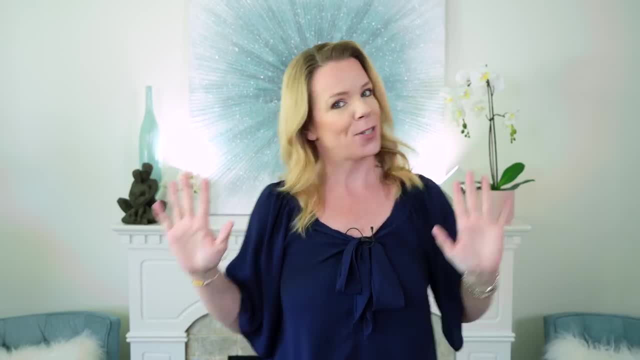 tricking your brain And the next thing you know you're doing the dishes and you feel happy about it. I don't know, man, It sounds crazy, But don't knock it till you try it. So I hope you're up. 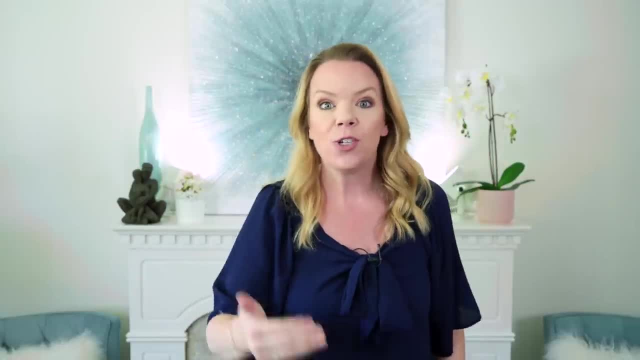 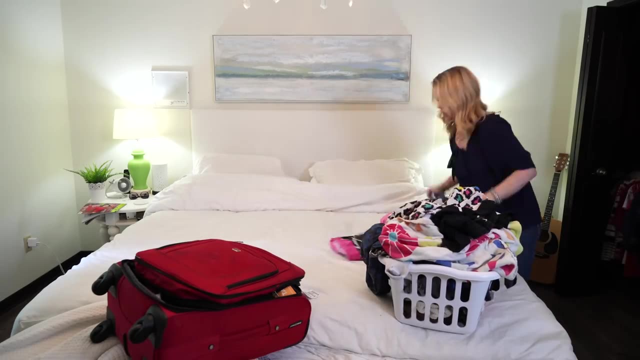 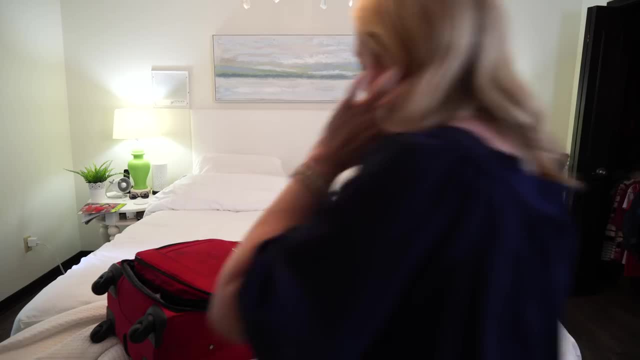 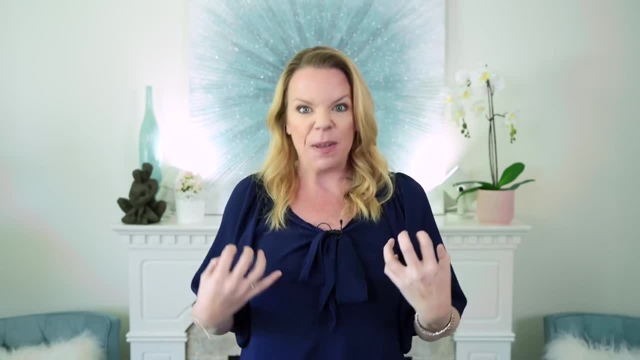 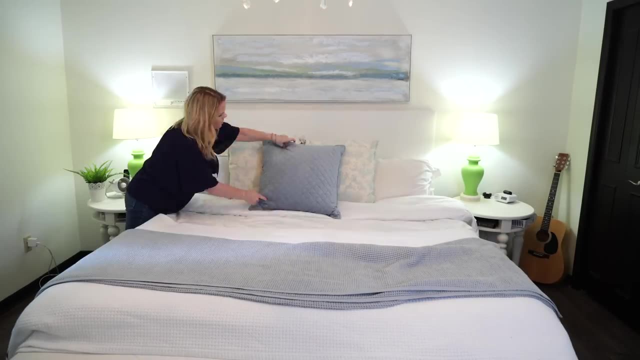 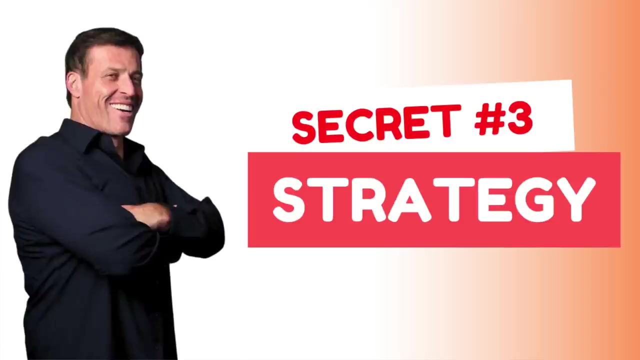 I want you to get up, I want you to feel excitement. fake the excitement and fake a new story, Because you're going to feel it working and you're going to actually want to clean your house. And the last part, the last trick, is strategy, And that means actually having 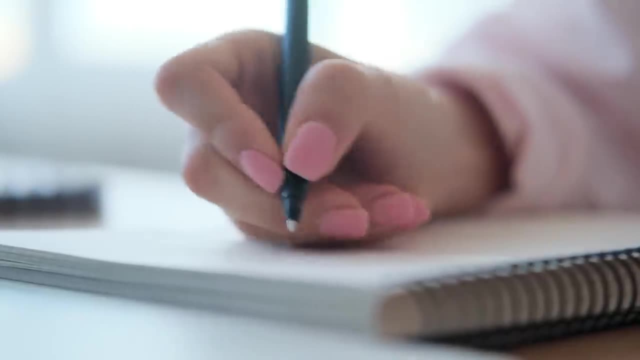 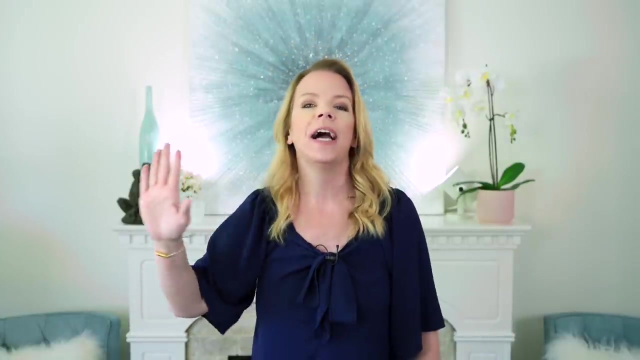 a plan, And this is simple as printing off a cleaning checklist and checking it off, And we always think that it's the plan that's going to get us there, the strategy. If only I could find the perfect cleaning schedule. or if only I had the perfect step-by-step solution. 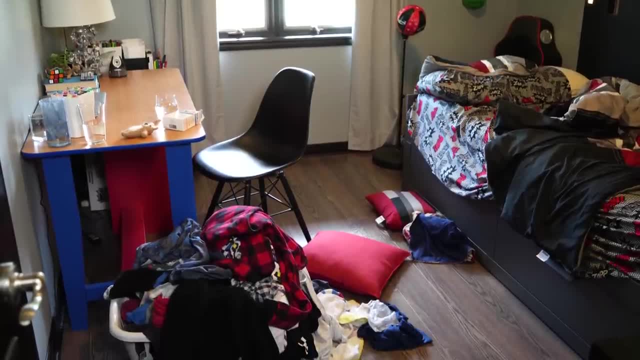 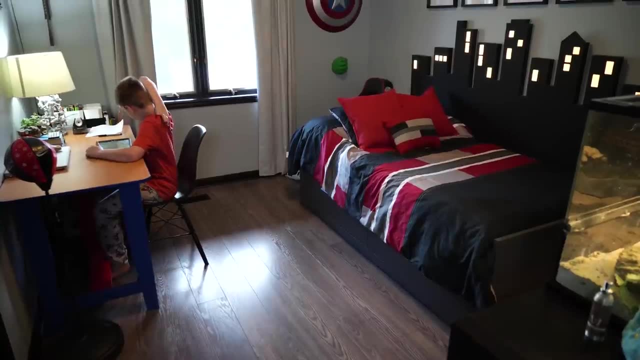 but that's the least important part. If we're in state, if we're like feeling excited and if we know we can do this and we want to do this, we don't need a plan, we don't need a strategy, but that does help. 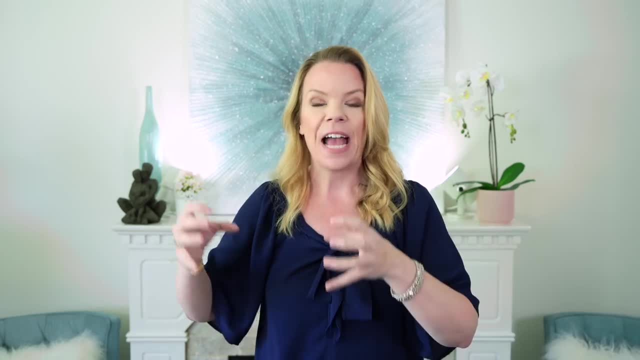 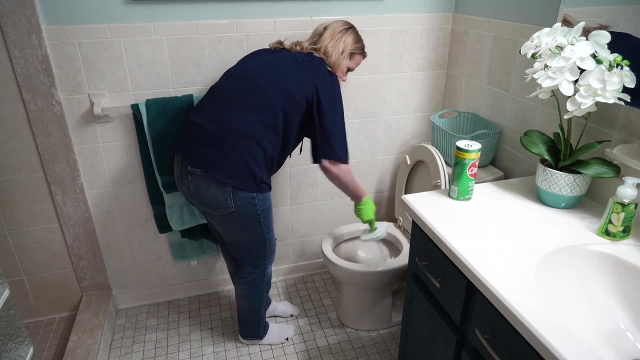 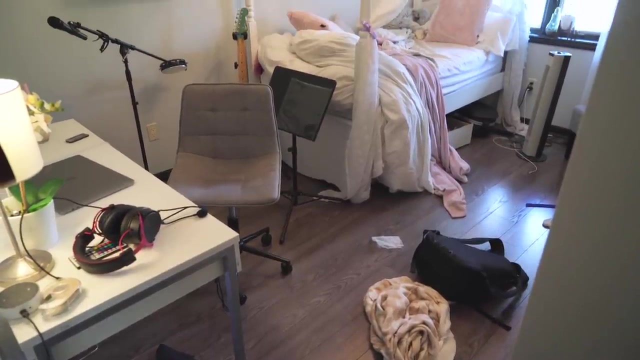 So when you combine these three things- the state, the story and the strategy- you can feel motivated to do anything, even scrub a toilet. my friends, I promise you this works. My house is a disaster right now. I'm faking excitement to clean it. 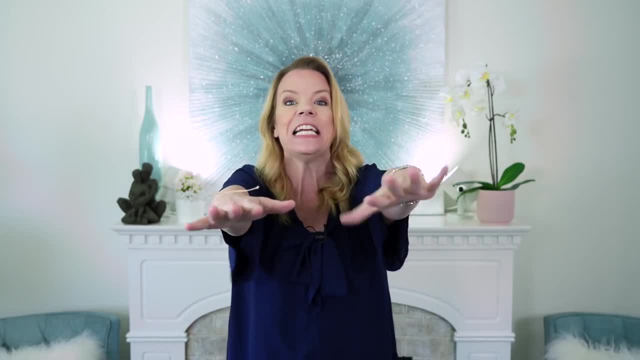 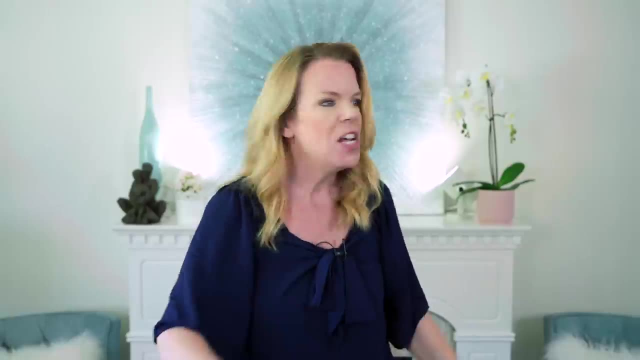 and I'm going to get there And I'm hoping you're doing the same thing, So we're going to clean together. right now. I want you to look around your home. pick something that you want to do, that you deserve to have done. 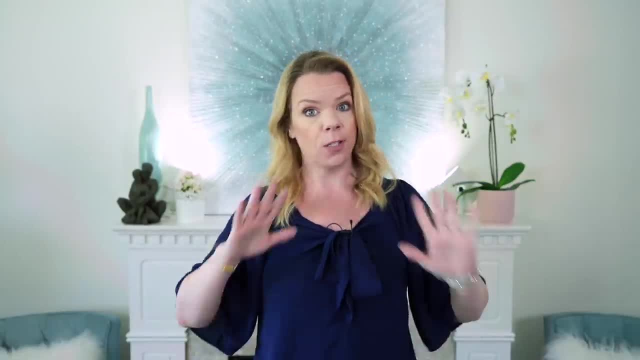 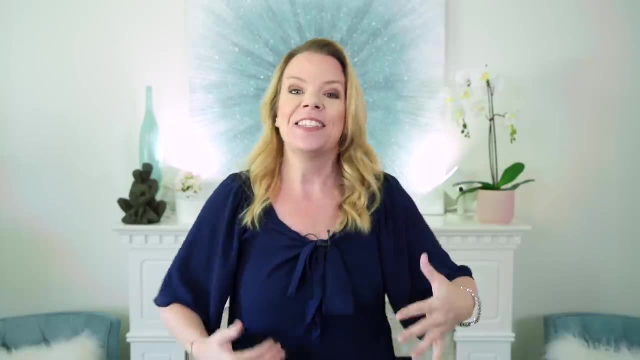 something small: a clean counter, wipe your bathroom, a sparkly toilet, whatever it is. Let's get up, let's start fist pumping, let's do some jumping jacks and let's tell ourselves: enough is enough, I deserve this. 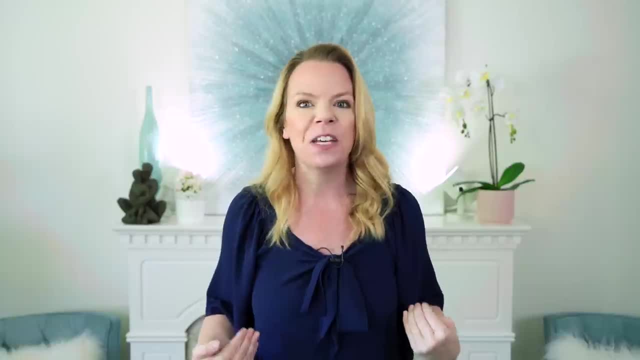 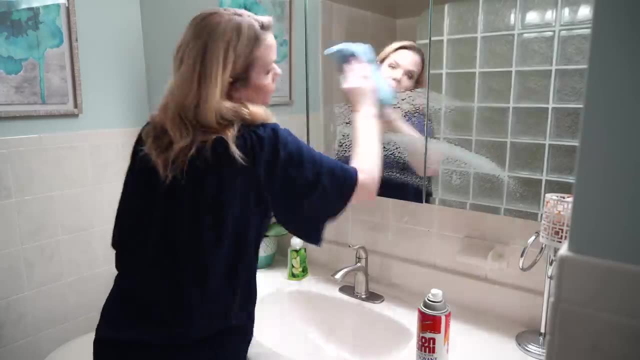 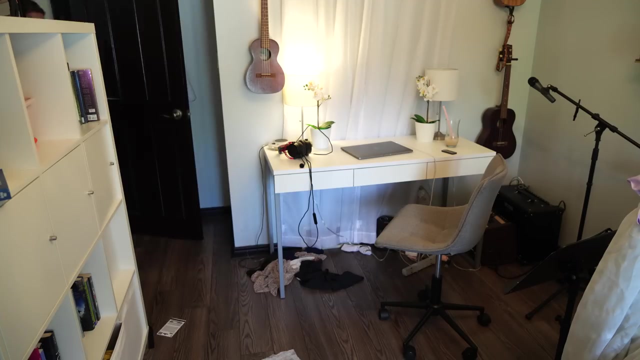 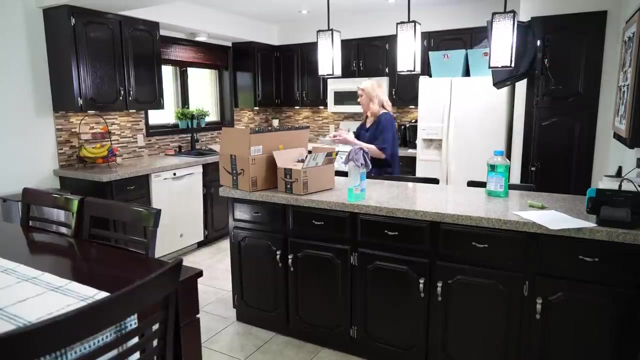 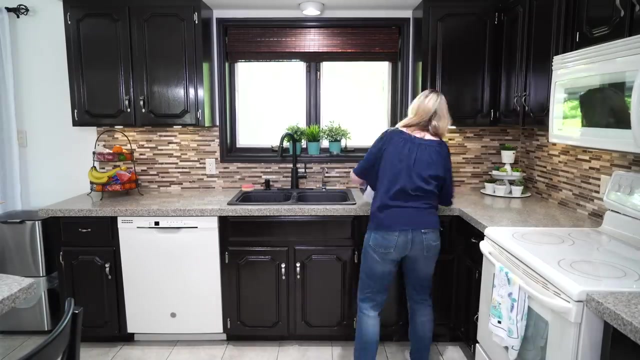 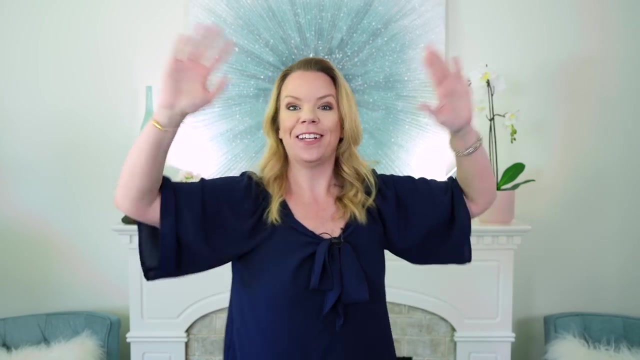 This is a gift to myself, because I'm going to feel amazing when I'm done. You feeling motivated. Let's do this. Let me know in the comments below if you actually got up, if you did a little woo, if you clapped your hands. 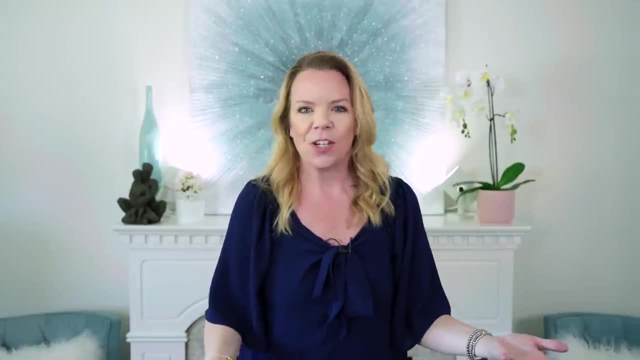 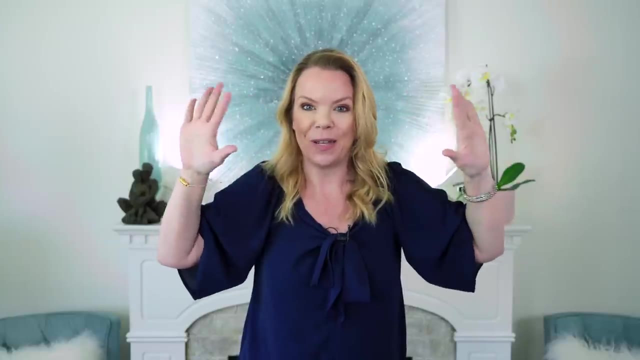 if you actually tidied something or if you passively watched this video. I'm not judging, I'm just curious because I know this can be uncomfortable. I remember the first time doing this at this Tony Robbins event. I was mortified. 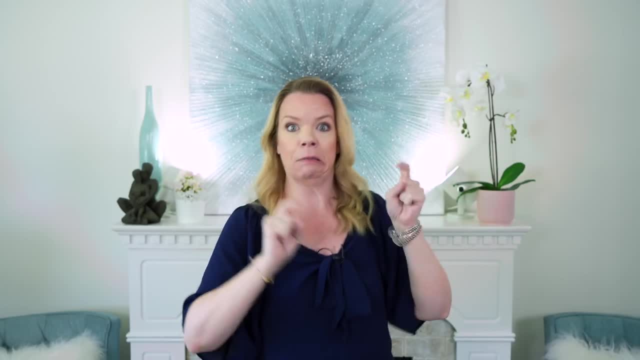 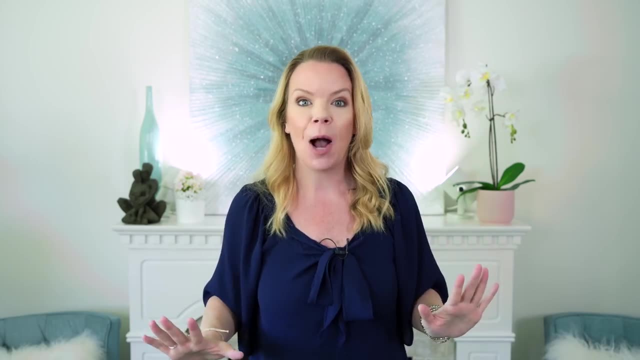 It felt like I was in a Zumba class. you know where you're just like do, do, do, do. I don't wanna do this, I feel uncomfortable, But it worked. it worked. So I'm curious. let me know in the comments below. 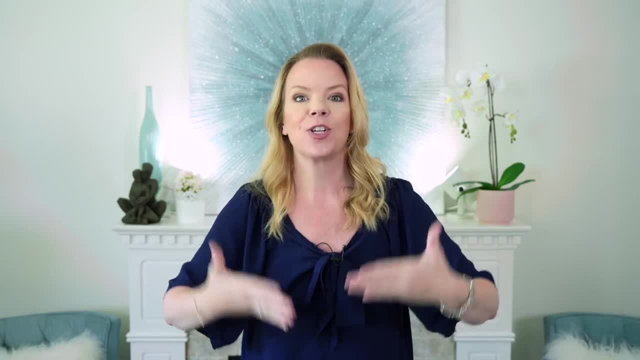 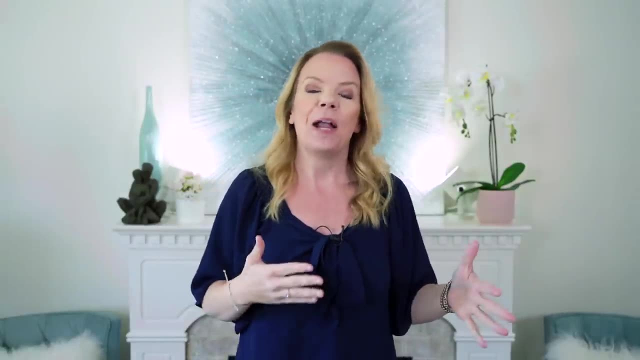 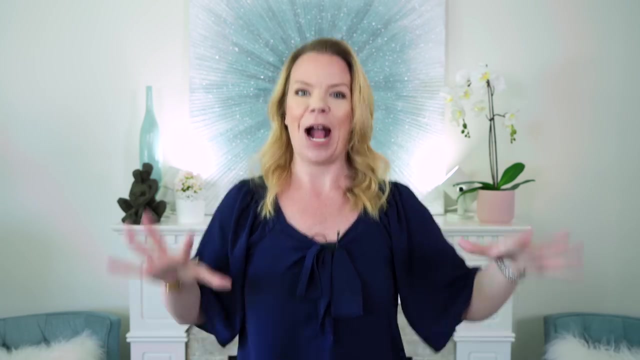 if you felt motivated, if you got up and actually used your body and used your words to trick your brain. I also want to let you know that I'm launching a 30-day organizing bootcamp that uses these strategies today. It starts today. 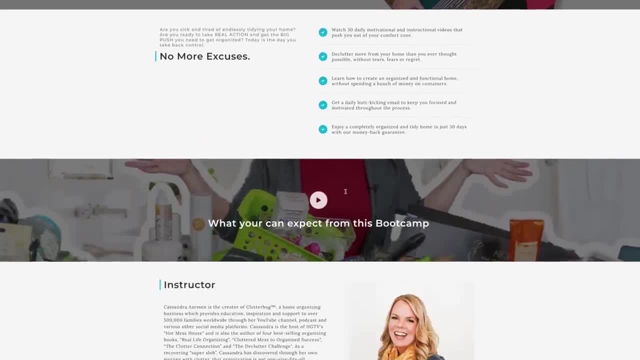 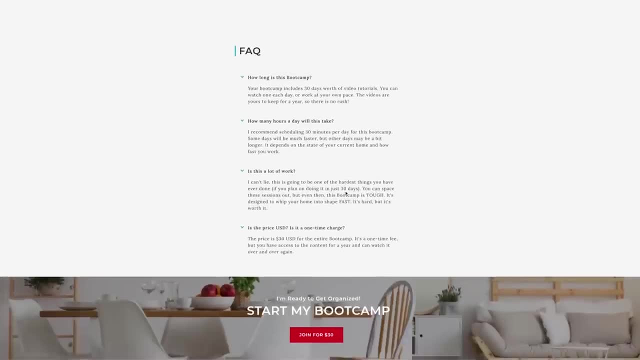 I'm so nervous- but I'm gonna put the link in the description so you can learn more about it- where I walk you through every single space in your home and I up your energy, I put you in state, we change your story and I give you a strategy for success. 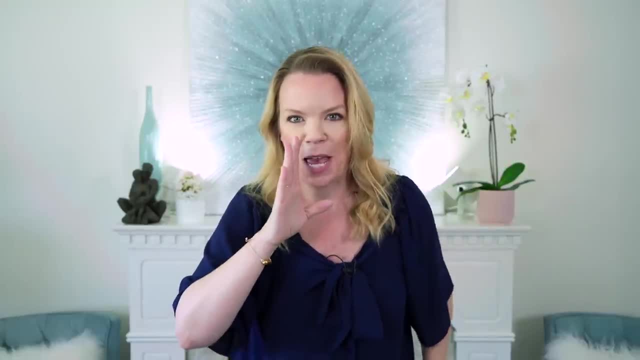 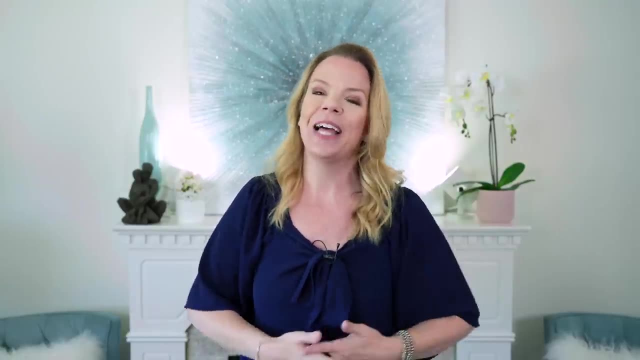 If this was cringey for you. you probably don't want the bootcamp, But if you feel motivated and you want more, check out the link below. And thanks so much for watching. I hope you liked and I'll see you guys next time. 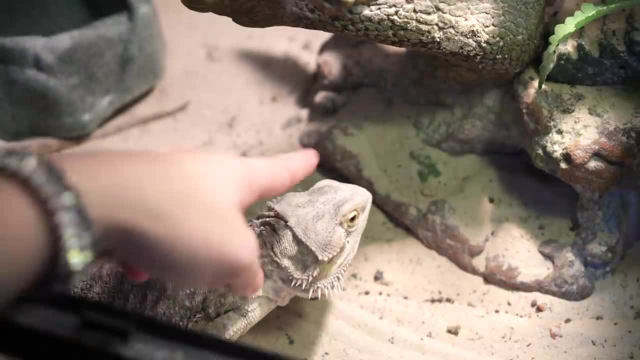 Thank you, guys. so much for those of you who have stayed to the end. We have a bearded dragon named Daenerys Targaryen, because she's a bearded dragon and I love, you know, Game of Thrones, But that's not the point.